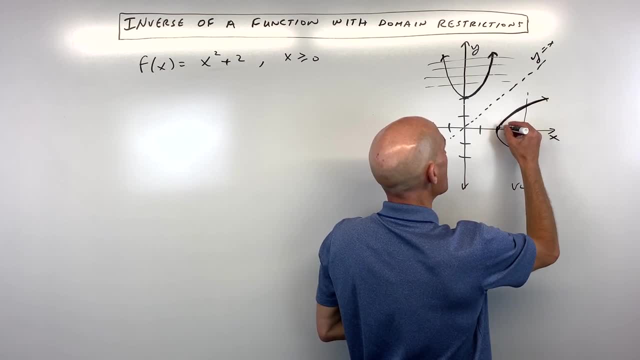 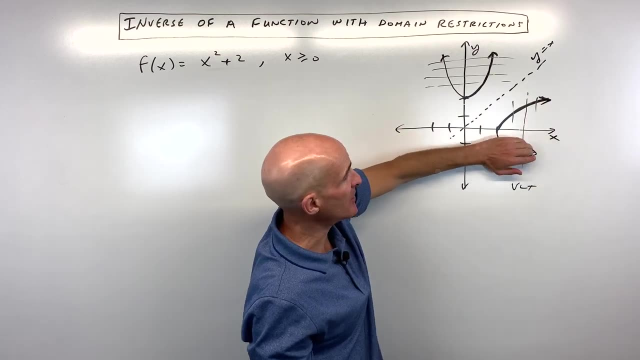 reflect it over. we're just going to be looking at this part of the graph- okay, the top part- and this does pass the vertical line test. It's only crossing at most once, So that means for every input there's only one output. 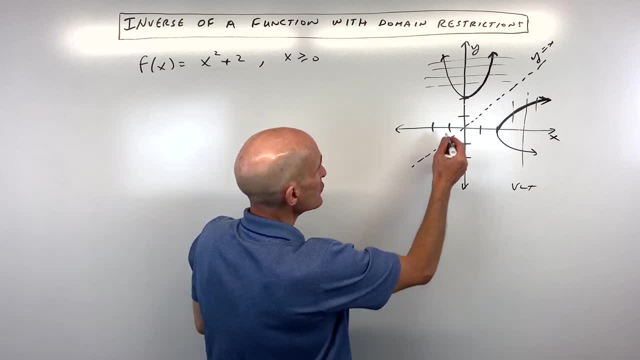 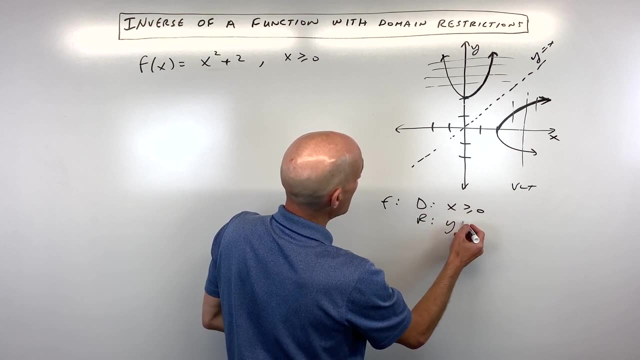 Okay, the next thing I like to do is I like to look at the domain here. So the domain of the original function is what x is greater than or equal to 0, and the range is y is greater than or equal to 2, right. 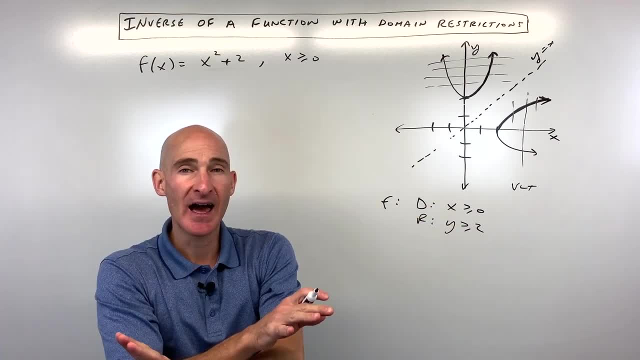 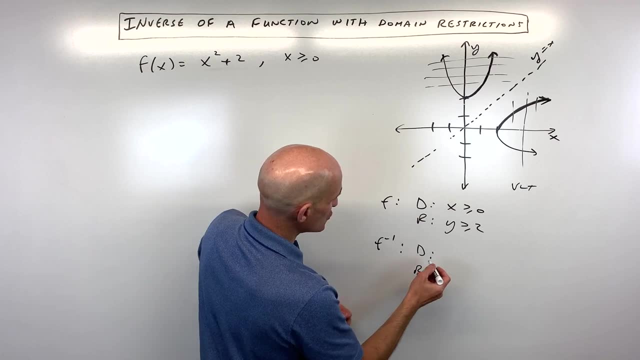 But when you find the inverse of a function, because you're switching the x and the y values, the domain and the range switch. So for the inverse, our domain and range switch. So now the range which was y is greater than or equal to 2,. 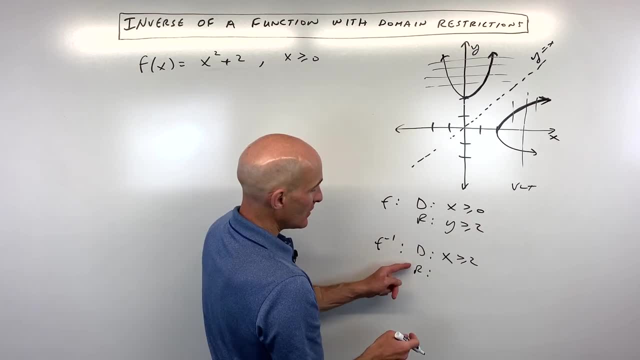 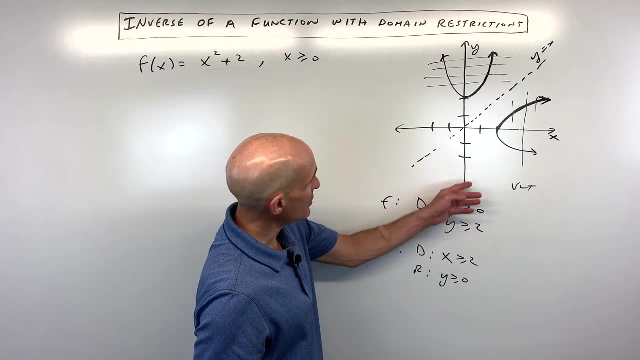 the domain is going to be: x is greater than or equal to 2, the range, okay, is going to be what the original domain was. So this is going to be: y is greater than or equal to 0.. So you can see over here on our graph: yep, that makes sense. x is greater than or equal to 2, and the range is: y is greater than or equal to 0.. 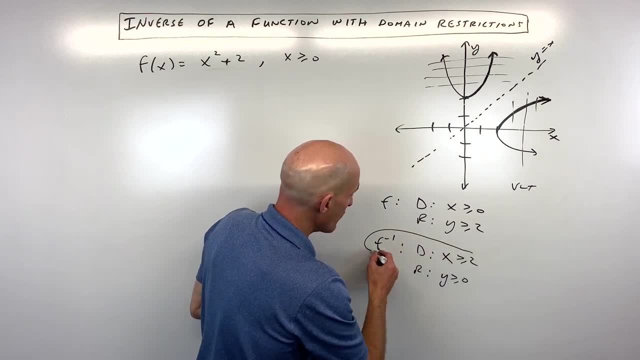 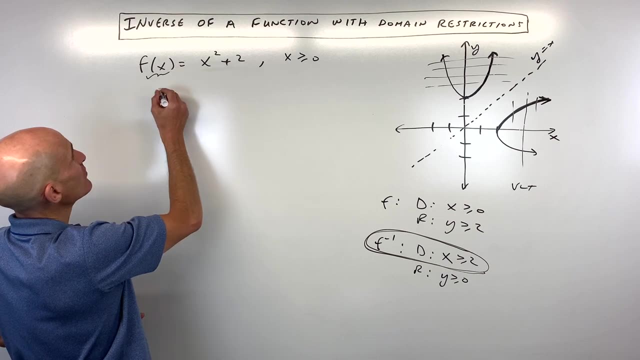 So they're just switching. So this is important because we're going to want to state this domain here when we find the inverse of this function. So let's go ahead and do that now. f of x. you can replace that with y. That's like our output. 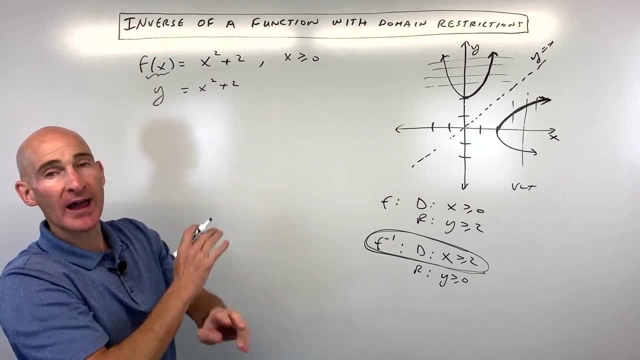 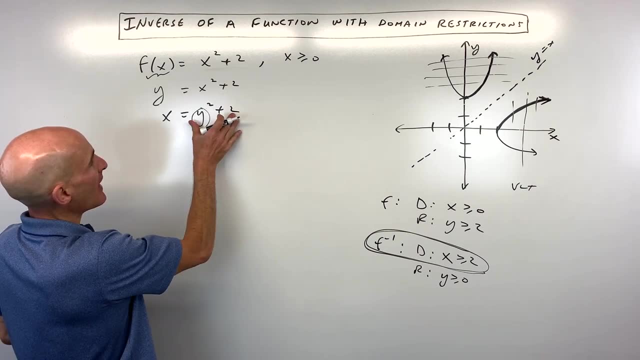 And now what we're going to do is, wherever you see x, you're going to put y And vice versa. So we have x equals y squared plus 2.. We're going to solve for the new y here Work from the outside in. We're going to subtract 2 from both sides. 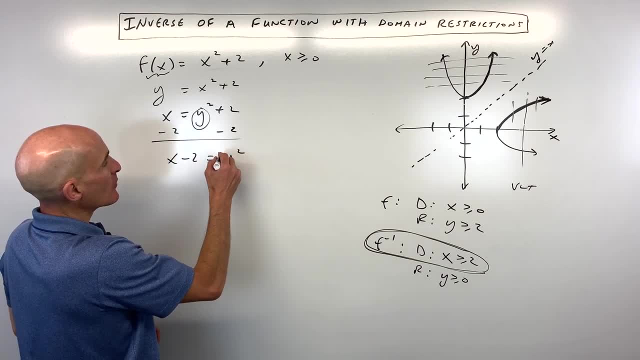 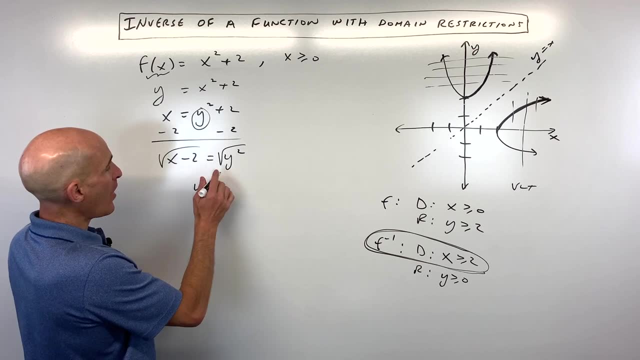 So we get x minus 2 equals y squared, And we're going to take the square root of both sides. Now remember, when you take the square root of both sides, you get two answers. right, We're actually going to get y equals, plus or minus, the square root of x minus 2.. 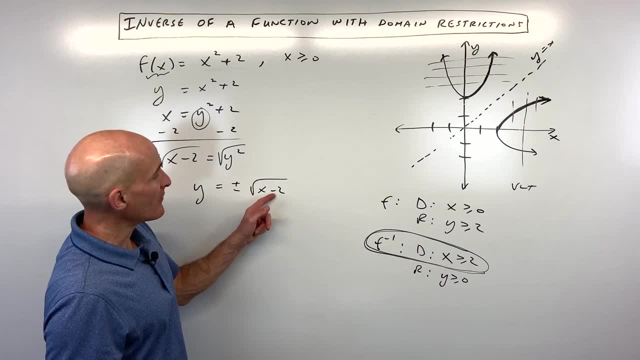 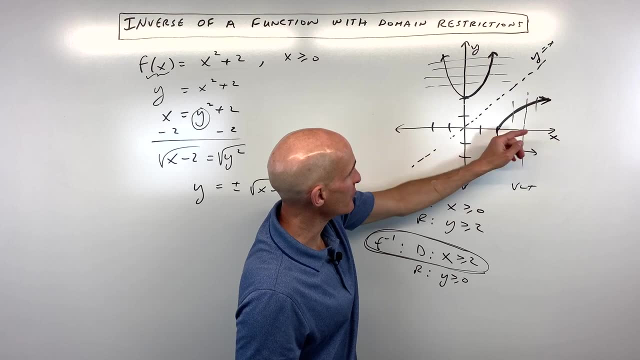 Now let's look at this for a moment. See: positive square root of x minus 2. is this graph right here? Negative times the square root of x minus 2, that negative is going to reflect it. That's this branch of the graph right here. 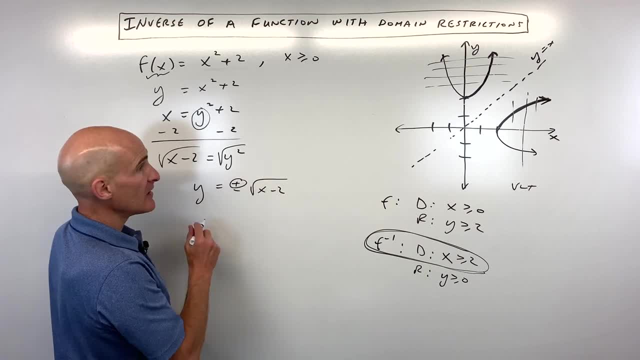 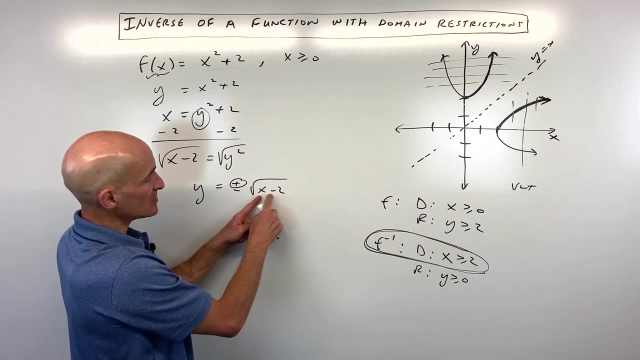 We're only interested in the positive one in this case, because of the domain restrictions. We want the range to be y is greater than or equal to 0. And we want the domain to be x is greater than or equal to 2.. And that makes sense as well, because you know if x is not equal to 2 or greater.